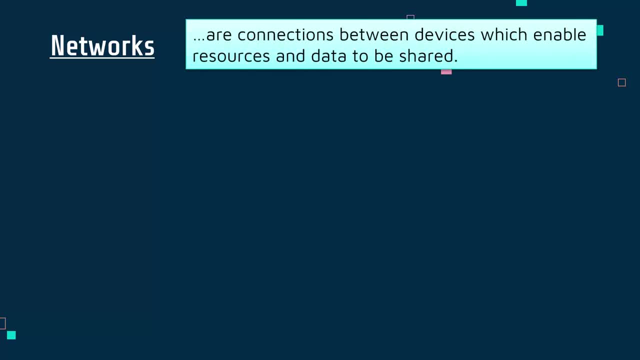 So network is the connections between devices which enable resources and data to be shared between those devices. So, because you are on YouTube watching this video, you're on a network- possibly your home network- which might be connected to the internet. maybe you are at school. 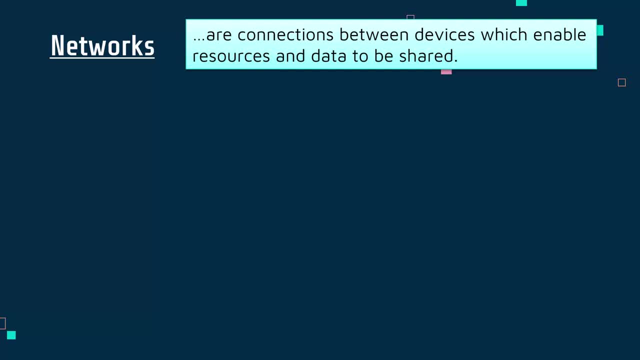 maybe you're on your phone. maybe you're using a personal hotspot If you connect wireless headphones to your phone. that's also a network: Any connection between devices which enables some data to be shared between them. So here is a relatively typical diagram of what a network 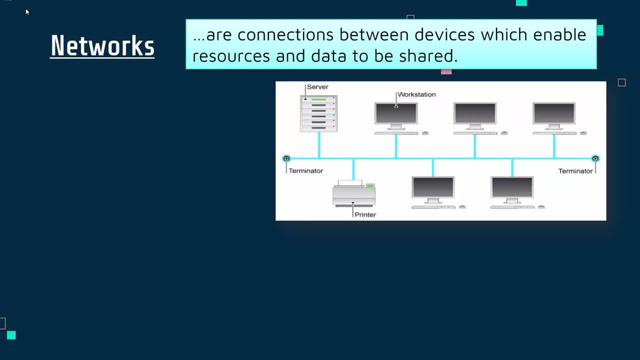 might look like. This is what we would call a bus network. We've got a big Y in the middle, which is what we call the bus, with computers connected to it, including a printer and a server, A server being a really powerful computer. Now, perhaps stating the obvious a little bit, but networks are important because they make 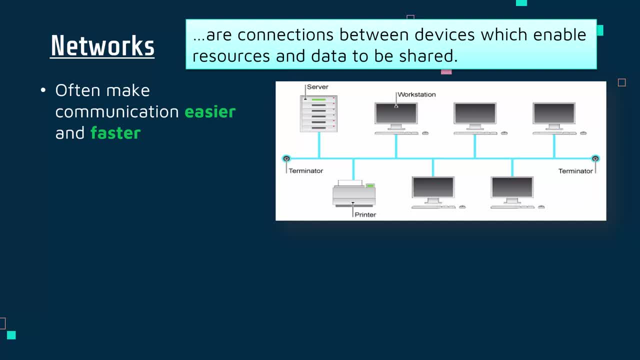 communication usually easier and faster. So, going back before networks were really around, if you say had an office in London and another office in Newcastle, you'd have to communicate via letter or via someone going between the two places via car or via train, Whereas now send an email over. 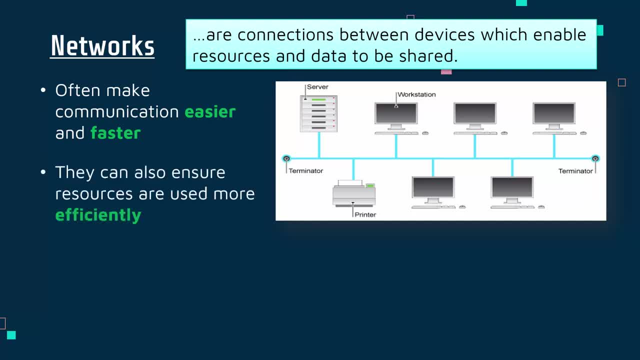 a network and it's much quicker and faster. Also, networks enable us to make use of our resources more efficiently In many cases. so in this network here we've got a printer, we've got a server and on our workstations we'll have some data and some software. All of those could be resources and having a network. 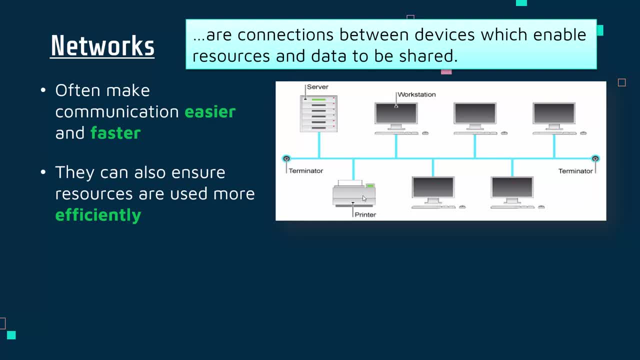 means you can share these more easily. So here I've got one printer connected to the network, and so every computer can use the printer. We don't need a separate printer for every computer, which is not an efficient use of resources. Now, an issue that can arise in most, I'll say, normal networks: 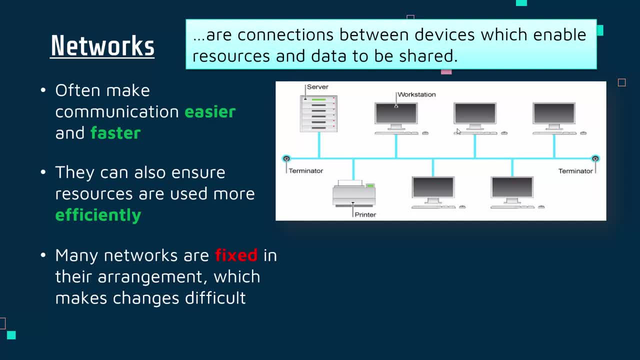 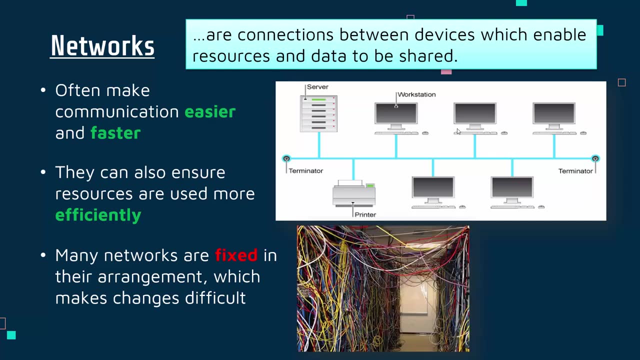 the ones you'll find at home or at school or in your home, is that you don't have enough resources. So if you want to make any changes, they're going to be quite difficult. Now, this image here will strike fear into any network administrator. all these wires crisscrossing Now, I hope, your school. 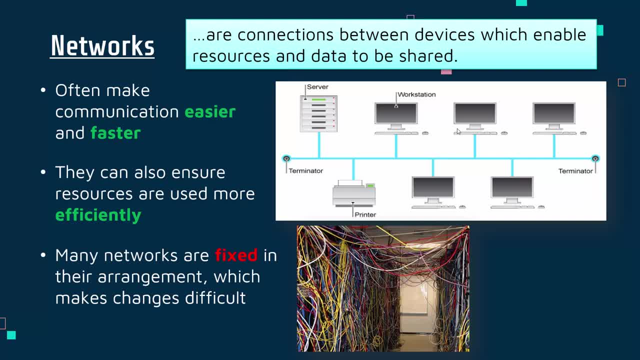 your home does not look like this, but the point remains: if you want to move one of your devices around, maybe you want to change where your printer is. if you want to move a server, it's not easy. So if you want to move it for 10 minutes, it's just not worth the effort to. 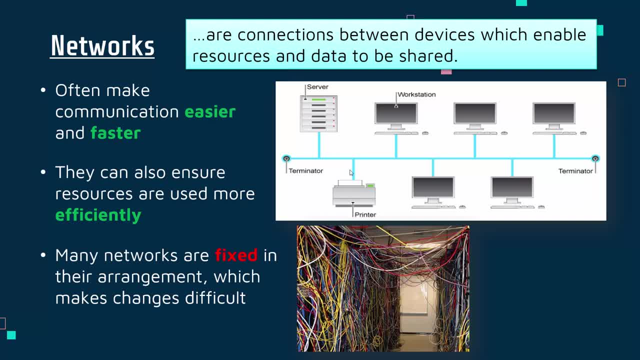 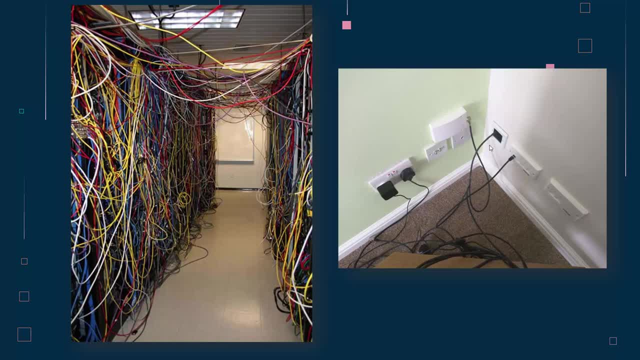 have to re-root all the wires and drill through a wall and all these sort of things. Even in a home, which is hopefully more reasonable, you've got certain ports in the wall where you plug in your router, plug in your TV, and it connects to the wider network. Now they're not everywhere, right? 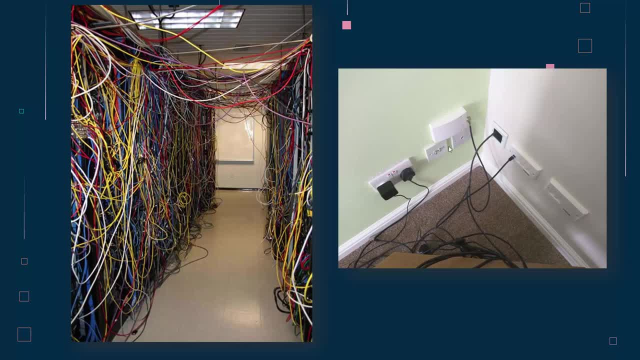 you probably don't have one of these ports in every single room of your house. there might be one room in your house which has these ports, and so your choice of where to put your router is not really a choice. I suppose you're kind of forced to put it. 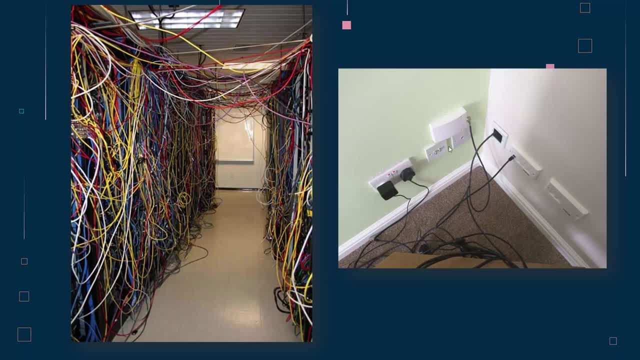 in a certain position And that lack of flexibility is okay most of the time. but if you want to make a small change, especially a temporary change, it's very hard to have to re-root and change the layout of your network. Let's say it's a beautiful sunny day and you want to go and work in your garden. 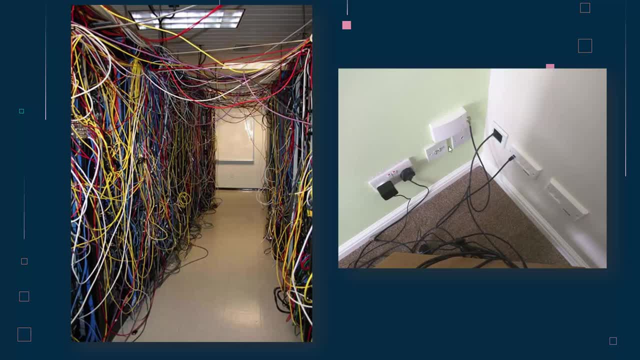 and your wireless router doesn't have a range big enough for you to to work in your garden on your laptop. Well, there are a number of ways that you can do that. One of the most common ways is to go and re-root your router. The issue is you can't easily just take your router outside because it's got a wire. 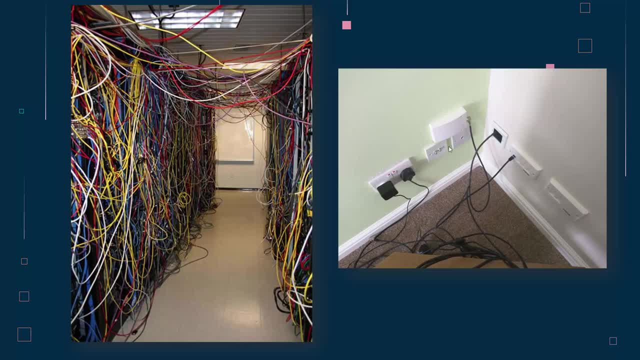 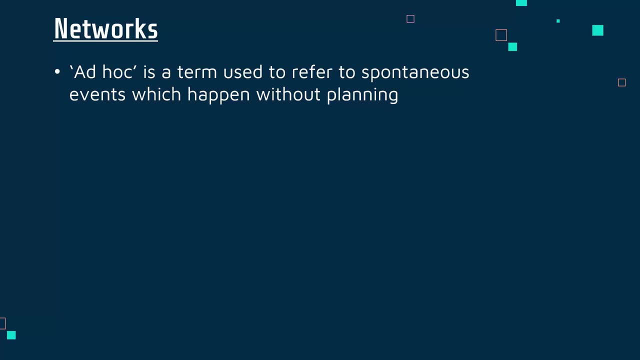 it's connected to the wall. it's not designed to just be moved around. it's meant to sit in one place in a fixed arrangement, And that lack of flexibility can be a problem and is why we have ad hoc networks. Now, if ad hoc as a phrase sounds a bit odd, it's because it is. it comes from Latin. 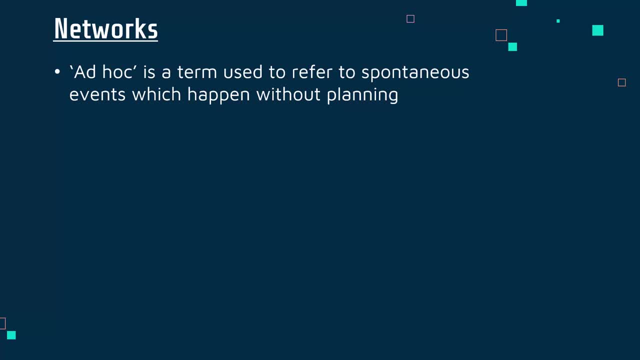 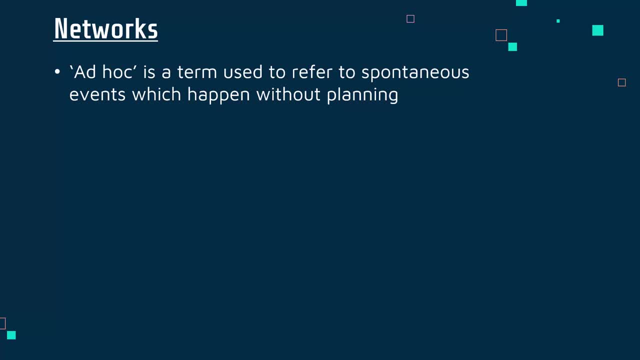 Now, ad hoc networks are similar in nature in that they're not really long-term solutions. They're networks which can be set up quite easily and can be flexibly changed, unlike most normal networks, and they're often set up for only a short period of time, so they're